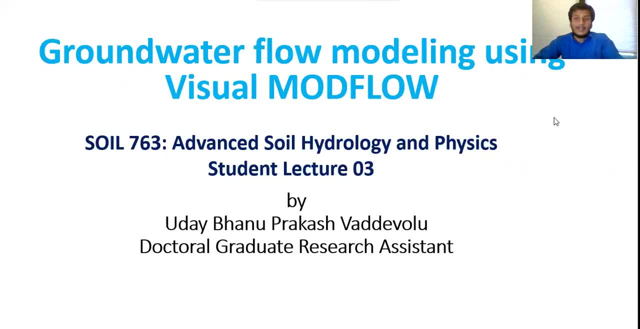 And try to explain the try to show the visual mode, flow software and groundwater modeling, And the outcomes would be like how they derive the partial difference, partial difference equation for finite difference model. And trying to- yeah, trying- to show the visual. 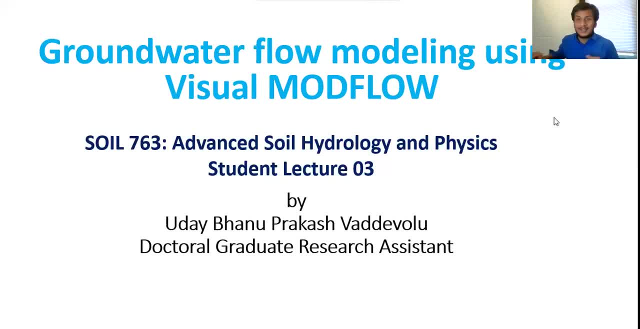 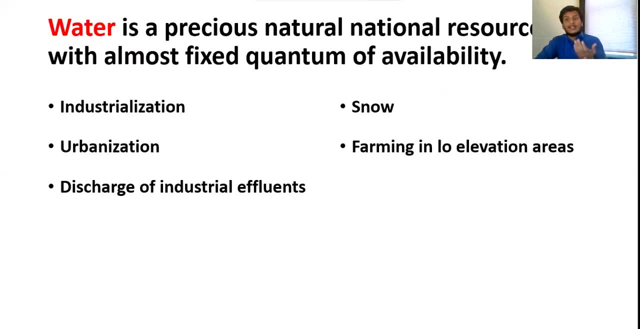 mode flow, So I hope everything will go smoothly here. So water, so in this nature, water is one of the most precious natural resource, which which is very important for us. So this on the on this earth. so we have different regions and different problems. Each region has different. 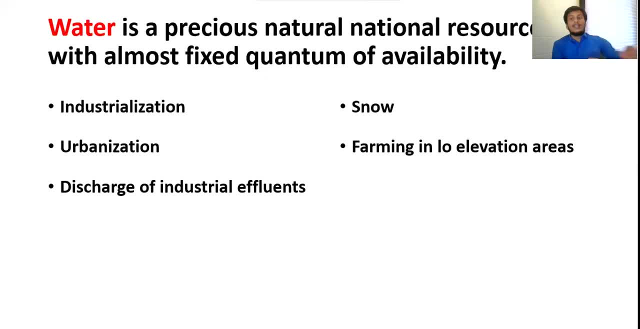 climatic conditions. Okay, We take an arid region. Arid region has more population, more like. the problems are related to water deficit. Like we do, they don't have like in these regions. water scarcity is one of the like major problem becoming major problem because, from last 15 years, Illinois and Lanninow 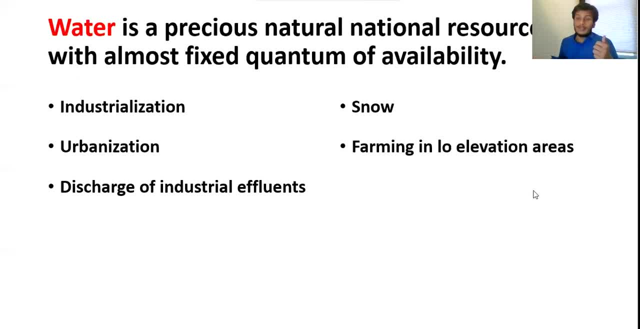 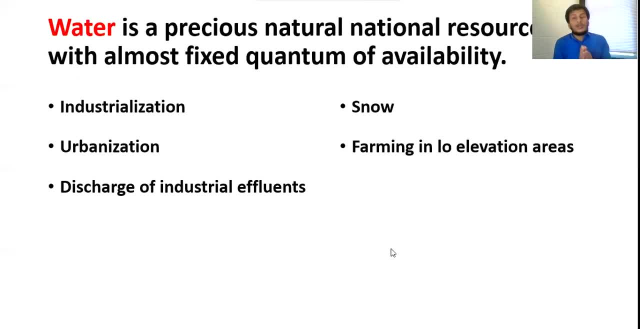 and other climatic conditions. So this is like we don't in some regions. most of the Asian continent doesn't have proper rain, proper rainfall, you know Which, which leads to reduction or decreasing in available water, And so, whereas people are using groundwater as the alternative source, and which which 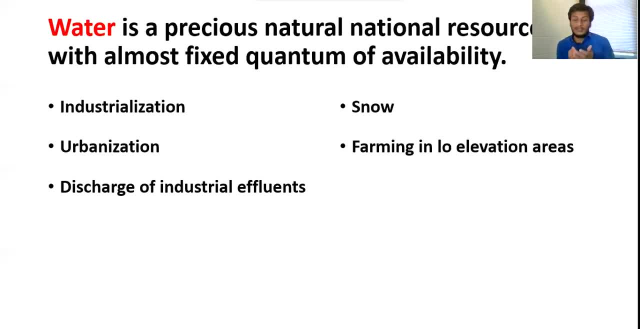 which is, which is, which is the only source of water that is available to the people? Yeah, And so, yeah, Okay, Thank you. alternative: but we don't have any recharge to the groundwater, so obviously the quality and quantity of the groundwater will go slow, slowly. so we need to, there is a necessity to model the groundwater. 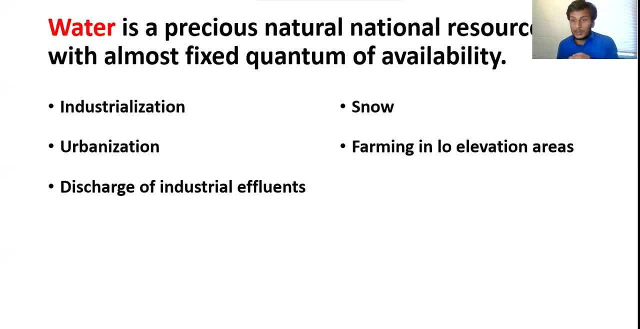 flow to, to, to solve to, to, to at least to know the water availability, to, to make the, to make the available water properly, to make use them properly. so, whereas in some other regions we have so far, and groundwater level goes up and downs, whereas like so, this very necessity for the 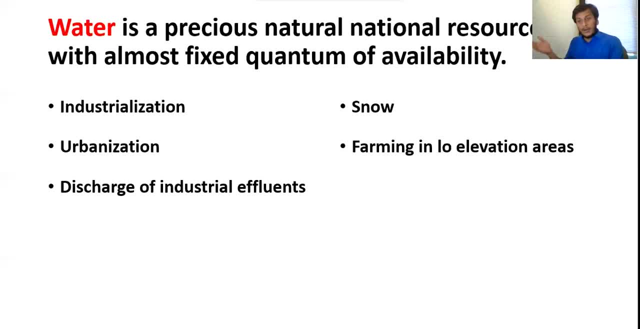 farmers, like farmers, are also interested in modeling them to know the groundwater level in their fields. so, yeah, this, this, this, this uh. so we, uh, we have certain softwares which which are used for groundwater modeling and all. so we are going to discuss the. so these are like kind of three. 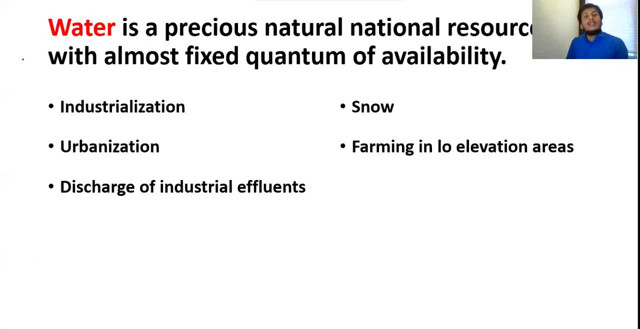 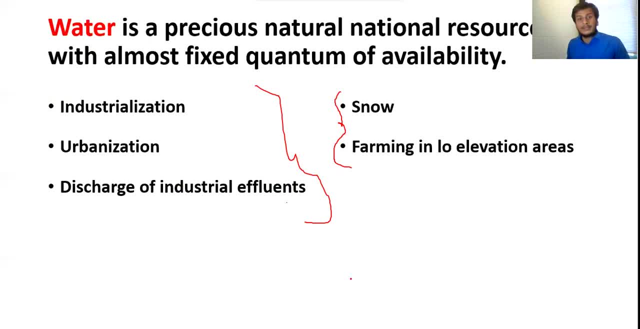 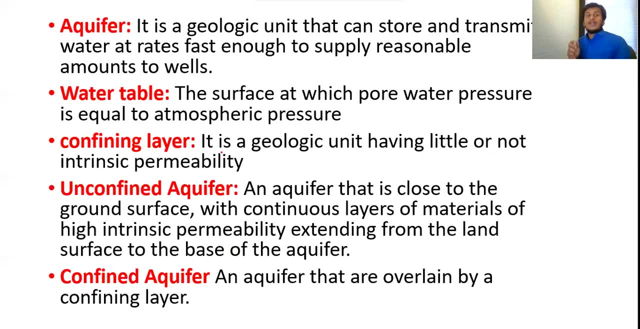 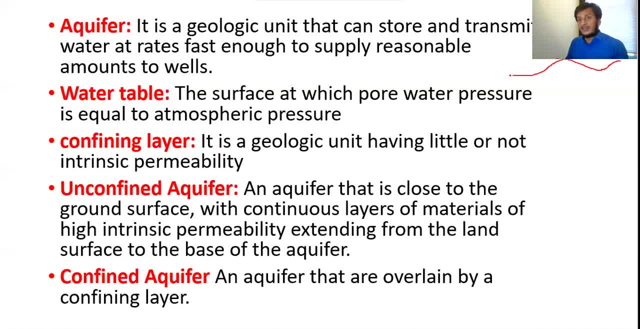 one surface water, we say surface. we have one surface water, we say surface. we have surface water. right, surface water, right, surface water, right. so suppose assume this is a surface water. so suppose assume this is a surface water. so suppose assume this is a surface water. this is sorry. assume this is a surface. 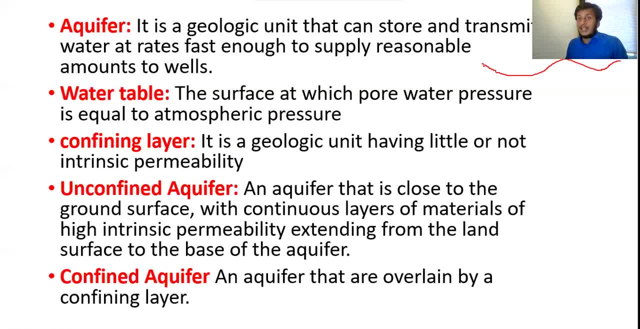 this is sorry. assume this is a surface water. this is sorry. assume this is a surface water. so water on the surface would. so water on the surface would. so water on the surface would. would flow. would stay on this, they won't. would flow. would stay on this, they won't. 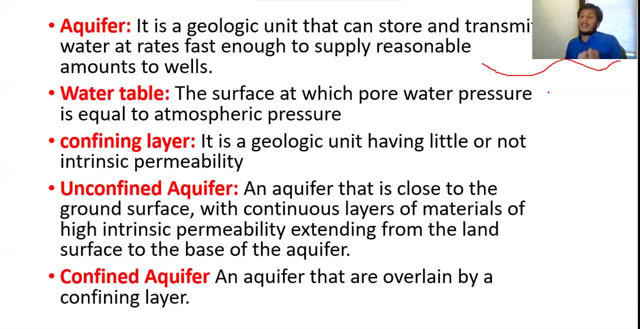 would flow, would stay on this. they won't. they will go beyond this, but they will go beyond this, but they will go beyond this, but with very low rate, very low, which with very low rate, very low, which with very low rate, very low, which causes infiltration and all. 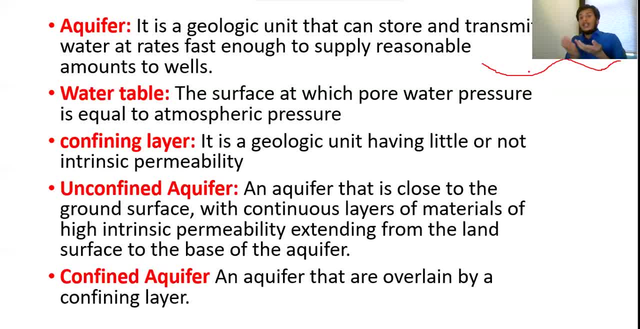 causes infiltration and all causes infiltration and all. so the the uh, so the the uh, so the the uh soil try to become an soil. try to become an soil, try to become an permeable layer. i would say permeable layer. i would say permeable layer. i would say it's not a permeable level, obviously it. 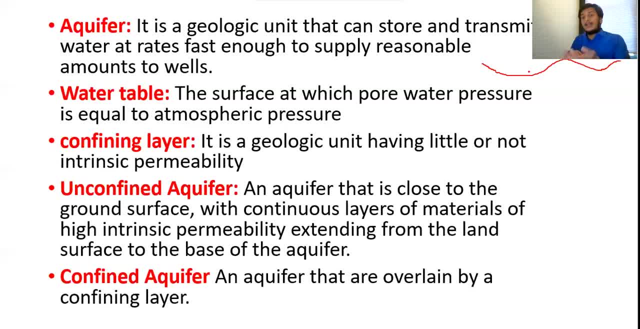 it's not a permeable level. obviously it it's not a permeable level. obviously it is permeable. layer is how water flows on the surface. water is how water flows on the surface. water is how water flows on the surface. water flows on the surface. so. 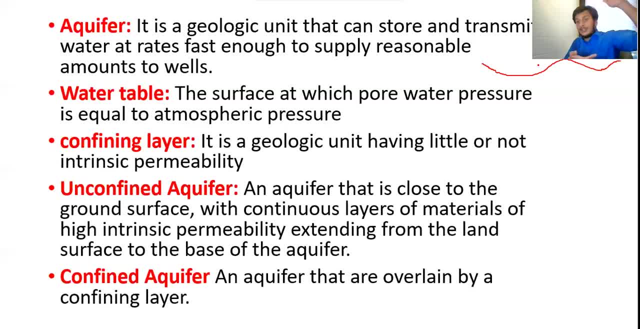 flows on the surface. so flows on the surface. so similarly in the groundwater in the, similarly in the groundwater in the, similarly in the groundwater in the surface, in the subsurface surface, in the subsurface surface, in the subsurface. if we say, this is the like, it is the. 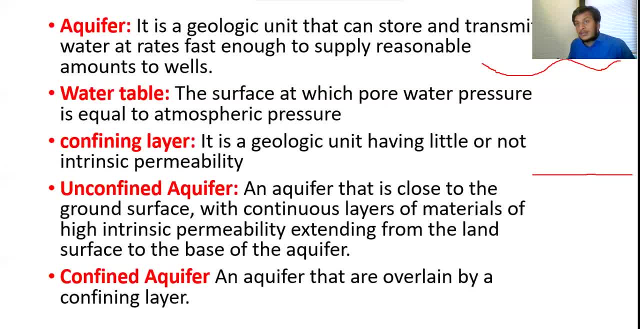 if we say this is the like, it is the. if we say this is the like, it is the surface surface surface, surface surface surface. this is subsurface which consists of. this is subsurface which consists of. this is subsurface which consists of soil. yeah, it consists of soil, right, yeah? 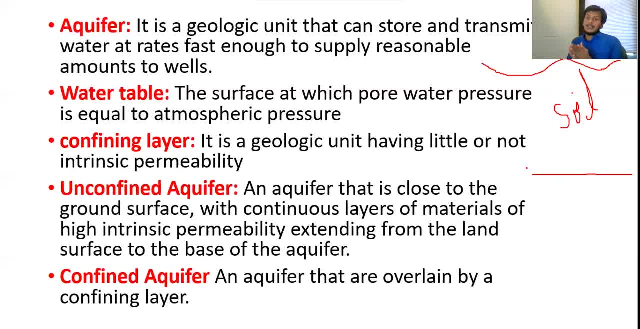 yeah, it consists of soil, right, yeah. yeah, it consists of soil, right, yeah, so we would be having uh, so we would be having uh, so we would be having uh same kind of things to hold the soil inside inside it, things to hold the soil inside inside it. 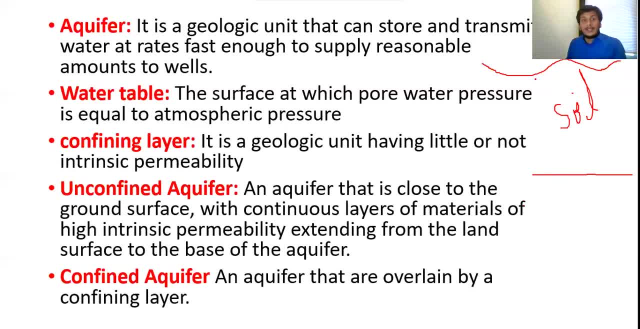 things: to hold the soil inside, inside it, to hold the soil, to hold the soil, to hold the soil, to hold the water. i'm sorry to hold the water, i'm sorry to hold the water, i'm sorry, so aquifer, so so aquifer, so so aquifer. so i'm gonna, i'm gonna explain few. 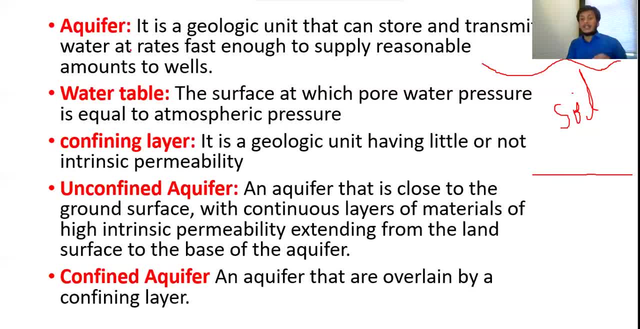 i'm gonna. i'm gonna explain few. i'm gonna. i'm gonna explain few properties inside the soil, which are properties inside the soil, which are properties inside the soil which are related to groundwater, related to groundwater, related to groundwater, aquifer. first, we say aquifer is a 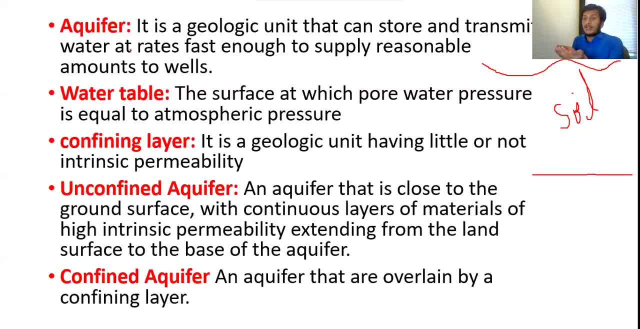 aquifer. first we say aquifer is a aquifer, first we say aquifer is a geological energy unit which will store geological energy unit which will store geological energy unit which will store some amount of water or some amount of water, or some amount of water, or transmit the water, which means it will. 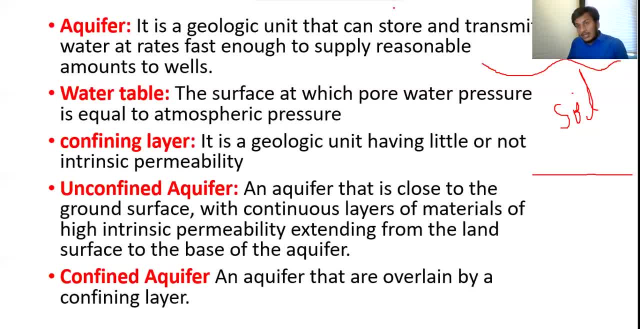 transmit the water, which means it will transmit the water, which means it will hold or hold or hold or it's kind of it's, it's a, it's kind of it's kind of it's a, it's kind of, it's kind of it's a it's kind of water on the surface. that is how it will. 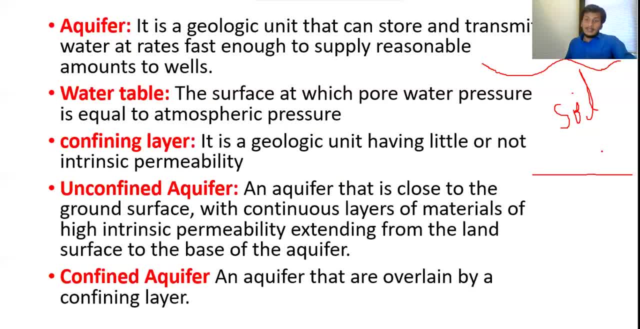 water on the surface. that is how it will water on the surface. that is how it will hold some water on the surface. hold some water on the surface. hold some water on the surface, similarly in inside the surface. that's similarly in inside the surface. that's similarly in inside the surface. that's what i'm talking about. 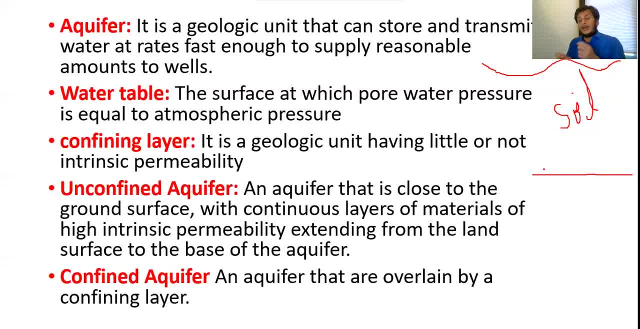 what i'm talking about. what i'm talking about, so this is called aquifer, so usually, so this is called aquifer, so usually, so this is called aquifer, so usually groundwater will start building like groundwater will start building, like groundwater will start building, like we can start. 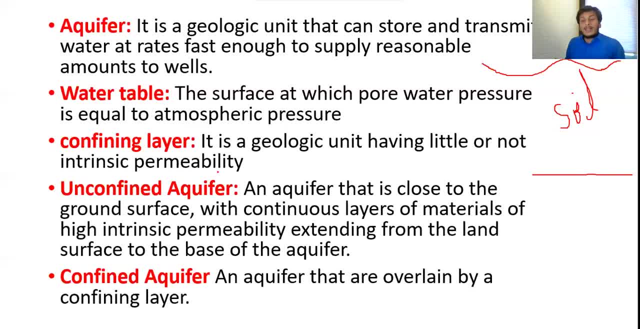 we can start. we can start from the, from the then water table. water table is the then water table water table is the then water table water table is the. we, i, i, i'm sure, like we are aware of it. we, i, i, i, i, i'm sure, like we are aware of it. 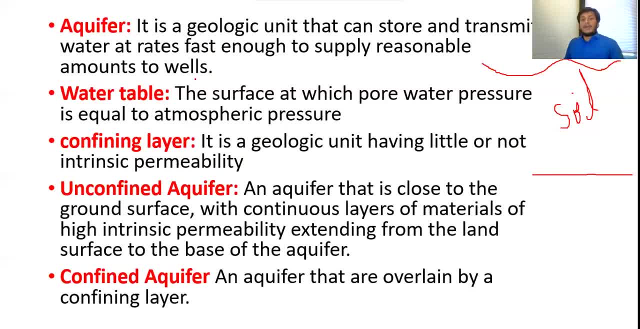 we, i, i, i, i, i, i'm sure, like we are aware of it, right. so what a table the the right? so what a table the the right? so what a table the the surface elevation of the groundwater, surface elevation of the groundwater, surface elevation of the groundwater level, or what is whatever. it is so. 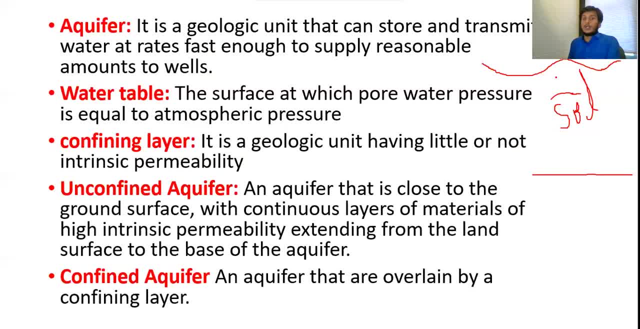 level or what is whatever it is so- level or what is whatever it is so, where it's pore water pressure is almost where it's pore water pressure is, almost where it's pore water pressure is almost equal to confining layer. It is a geological unit having little or not intrinsic permeability. That is what. 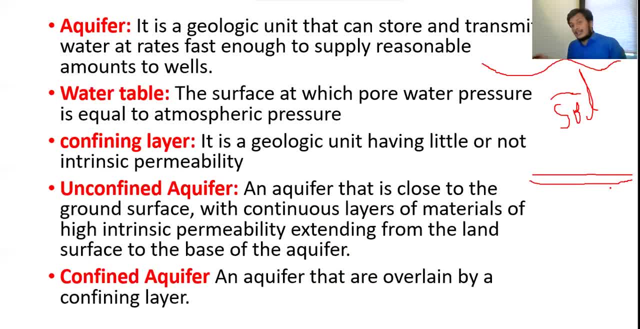 I am talking about. So usually aquifer has a boundary or as an impermeable layer which will not allow water to pass through it. That is called the layer, is called as confined layer. Usually groundwater will start going together, or I won't say going Groundwater will start storing on the 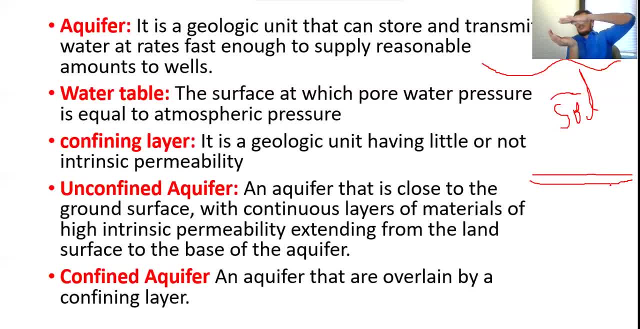 confined layer. Slowly, groundwater level will increase slowly. This is the confined layer because it can not go beyond this. This is called confined layer. Then comes to types of aquifers. We have types of aquifer, unconfined aquifer and confined aquifer. 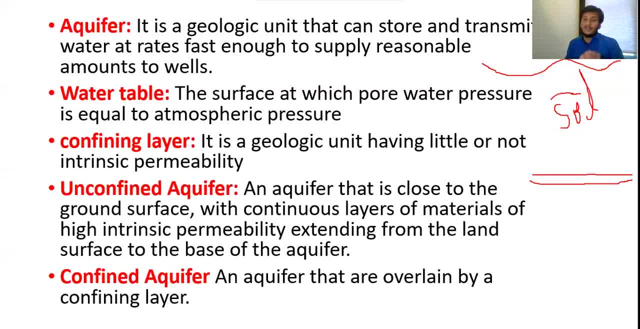 P перваяЕТ смотрите. We have types of aquifer: unconfined aquifer, confined aquifer. We have types of]. the third one is purged water table, which is you get with, like if it helps, so let's. let's see the. 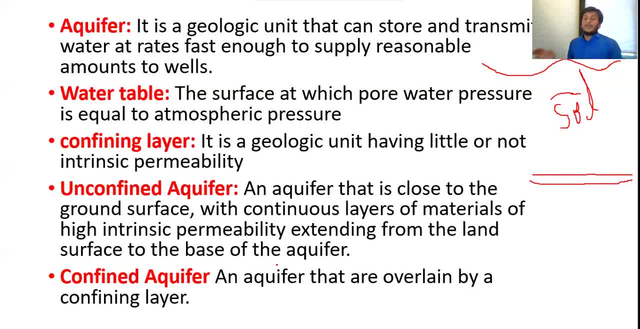 main policy: unconfined. unconfined it further. which or which is like uh, which is uh, most common? i would say yeah. so for unconfined identifier, there will be no like uh, no other confined layer above or below it which says like, which has less pressure of water compared to the other. 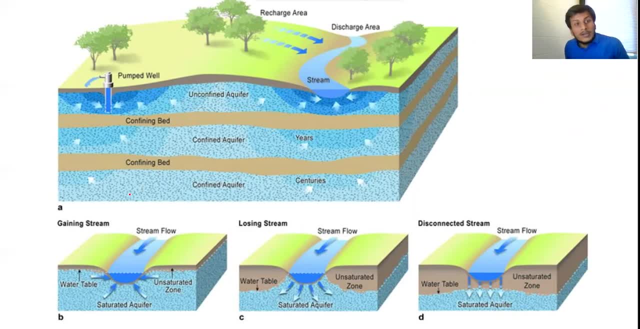 whereas confine liquid has two confines. in this figure we can see that. so usually this is what happens. this is surface water. we go. this is the base flow of some other flows like inside the surface, which would travel through towards the lower elevation. obviously, ultimately they will. 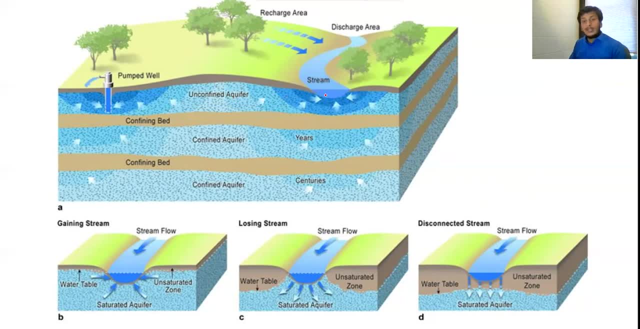 go somewhere. so, yeah, so this is the unconfined, this is the confining bed. this is the confining bed, which means water may not it it. most of the times, if they don't have any leakage, water won't pass through it. that is, that is how, like, we call. we call them as: 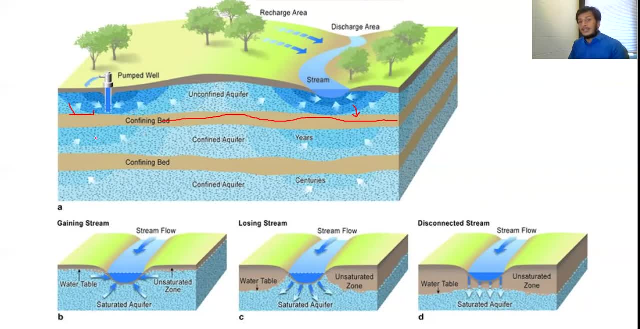 impermeable layers which would block the water movement. this, the water in this, on the above single confined layer, is called as unconfined. so this is the surface. this is not unconfined surface. so again, this is confined surface. this is complex. water in this region is called as confined. i mean the, the water storage in. 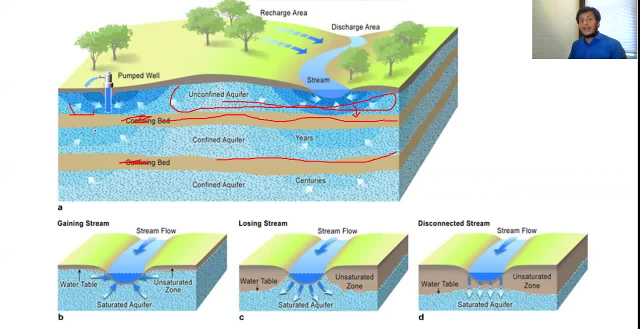 this region, the whole region, is known as aquifer. this whole reason pressure on aquifer is like bit higher than the unconfined. this is because water doesn't have any higher movement, because water is in pressure, because two confined layers are between, or the boundaries or acting as a boundary. 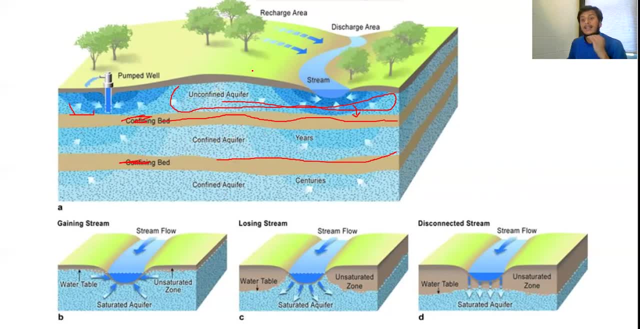 between the water. that is why they, they, they, they, they have like a higher pressure than the unconfined water in the unconfined. so we have a third type of aquifer which has it's called as leaky. leaky aquifer, which means like there's there would be leakage. 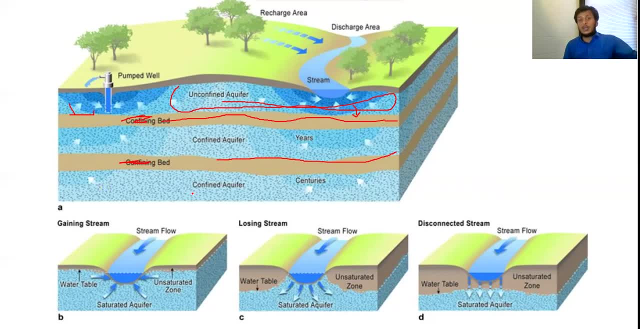 or kind of water movement through the confining, special case of confining. so this figure shows the, the, the, the uh uh gaining stream, some losing stream, how the water movement, how it's it's going here, it depends on the elevation of the disconnected stream, which is say slightly, yeah, these are like i just, i just got this. 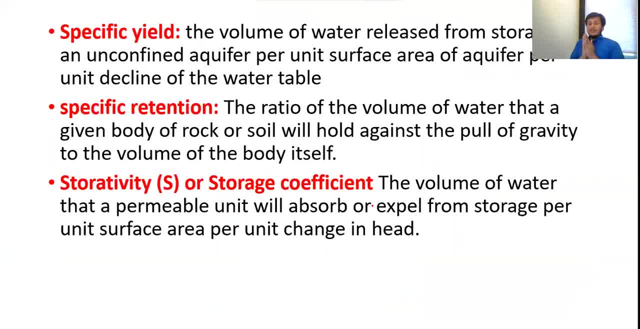 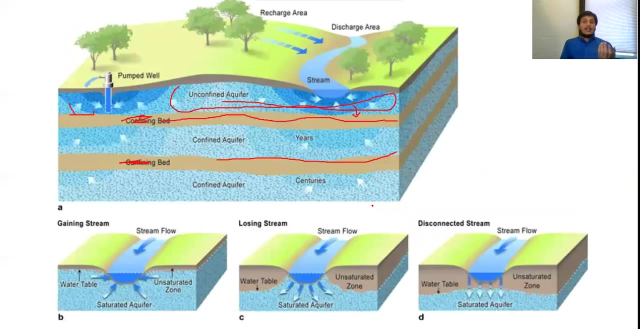 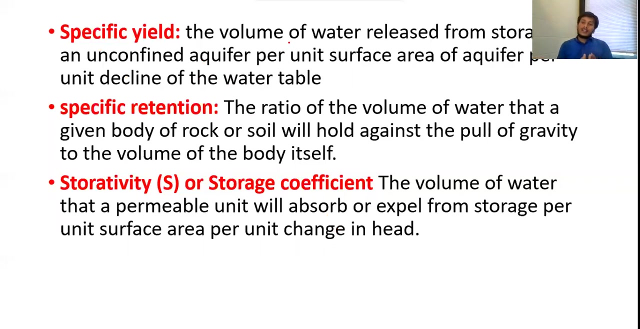 picture from internet. so let's discuss some uh properties of an egg: specific yield, specific retention, storage coefficient, transmissivity, high hydraulic conductivity, specific storage- these are some of the important properties of an egg which would say, suppose issue like that, yeah, specific field, obviously, amount of water released from the storage. 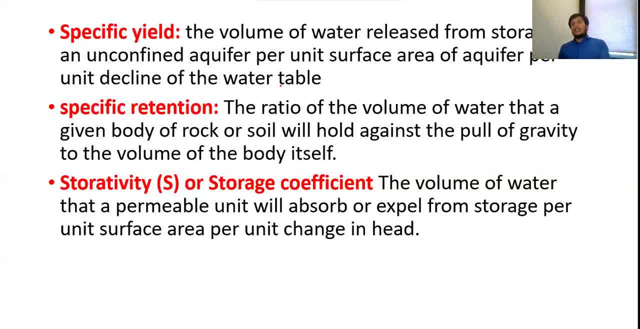 per unit surface area of the aquifer, per unit decline of the water table. if you can have water, this is called specifically group of water like will you know what you're talking about in terms of water released from the storage? then retention, obviously the name itself, how much soil it can take, how much water it can hold against. 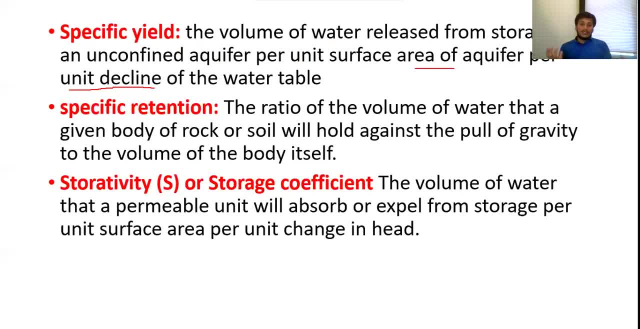 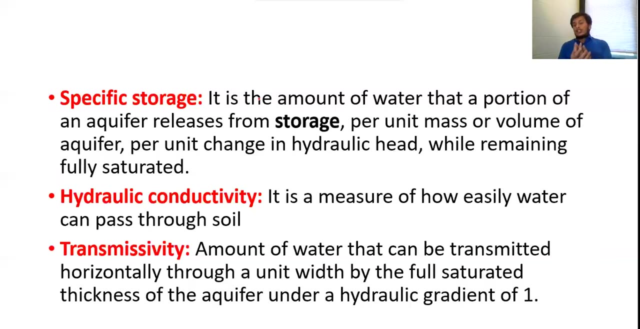 that is also a specific retention storage position. obviously, how much? how much amount of water is right to absorb from the storage part? storage that is, that is a store storativity or storage specific storage. it is the amount of water that was stored in per unit mass. i'm sorry. 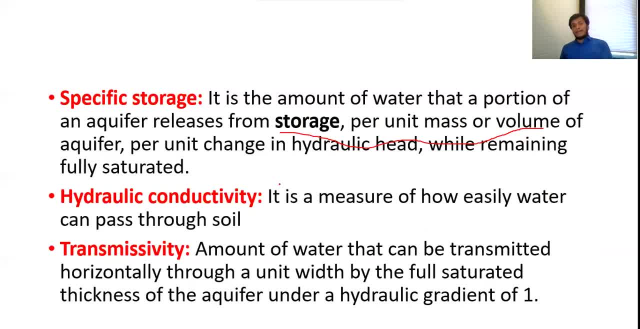 storage per unit mass or volume of it. this would say like: uh, the storage capacity per unit, per unit volume or something. hydrologically, this is the rate of flow of water, how the water flow in the, in the surface. assume this as surface. how the water, right we are. 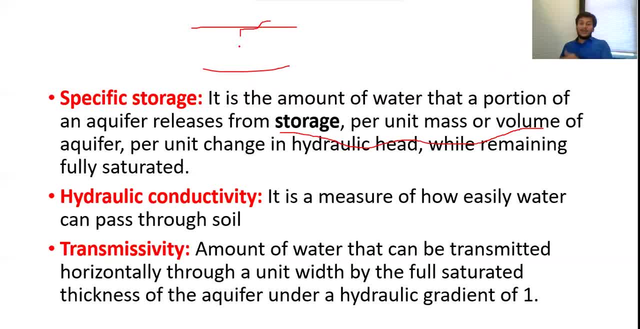 more aware of it, right? we always all saturated hydraulic creativity and all, etc. yeah, yeah, transmissivity, which is uh, can be transmitted horizontally through a unit, horizontal, horizontal movement, is transmissivity, hydraulic conductivity, so we would say hyper transmittivity. t is a equal to. 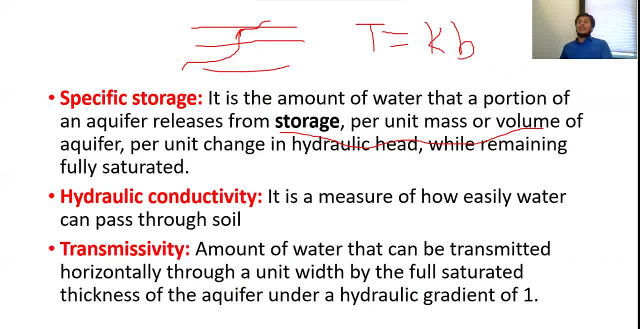 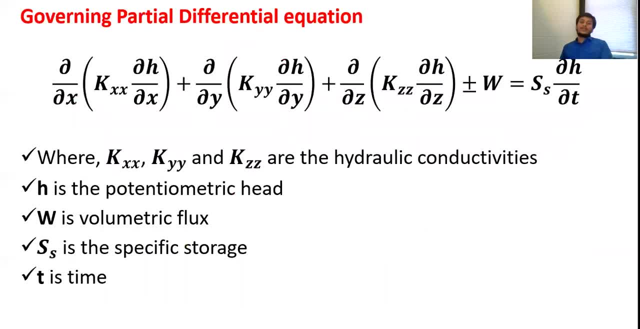 a into b, whereas b is the thickness of the aquifer. thickness of the aquifer, hydraulic conductivity into thickness of that. this is the transmission. so these are the properties, so usually any groundwater flow. obviously these are very important characteristics or properties to to monitor or track the groundwater flow. 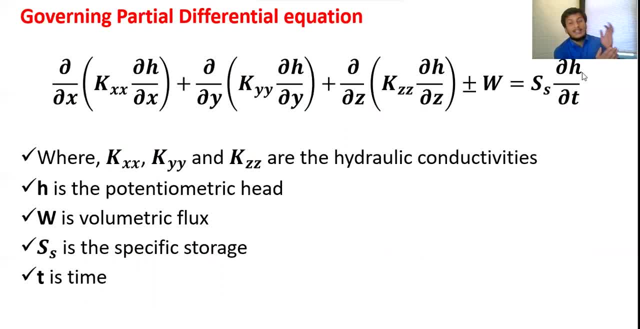 because we need all these properties, we need this. some of, at least some of them are very important to monitor or track the water flow. so this is a final governing partial differential equation for visual mod flow, which would say like, which would explain the hydraulic conductivity in x. 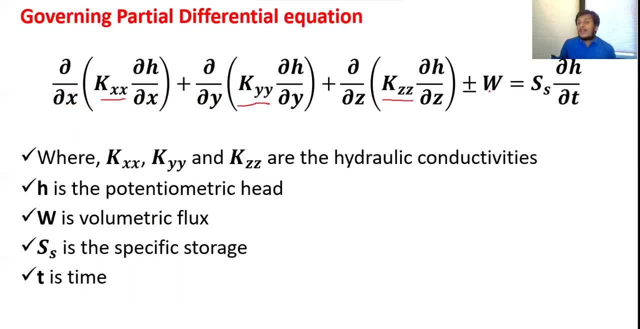 direction, y direction, z direction, then volumetric flux, then such, uh sorry, specific storage- i'm sorry, uh, it is a potential per potential metric head- then time partial differential equation which would like to, which is trying trying to explain us to the the water movement in each direction. it's trying to crack it. 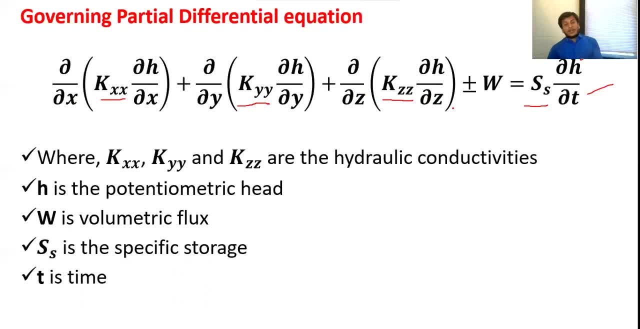 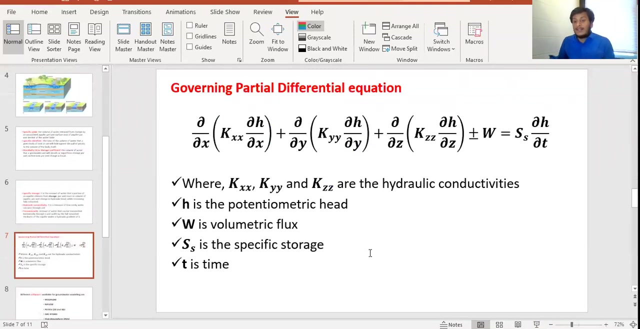 so, based on this equation, visual mock flow, startup, do the visual mode flow, i'd like to show some uh, some, some, some, some articles, books which worked on which, which worked on the uh partial differential equation, because, uh, i hope you guys are here in today's class like uh, by, by. 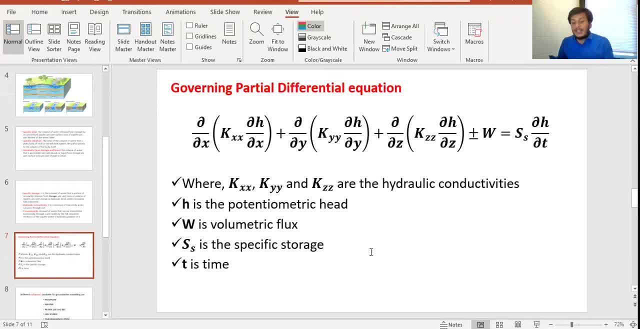 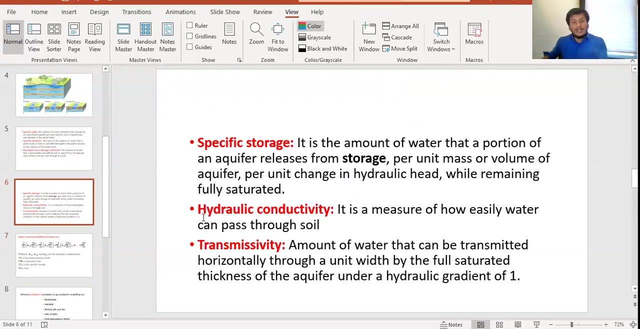 discussing about partial differential finite difference method and current elemental method in this class dr may help us to understand the uh, the, the this, how they solve the equations, how they use the mathematics, uh functions, transformations and all to monitor some, some hydrological properties and all. so i'd like to show a few things related to 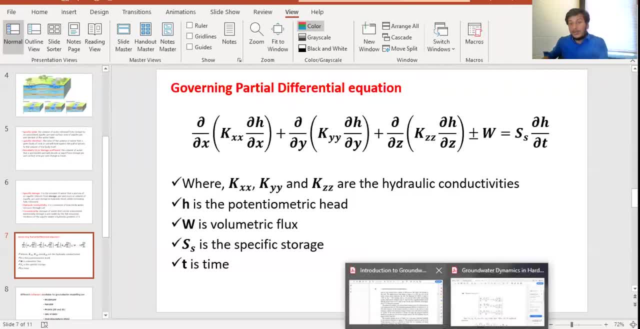 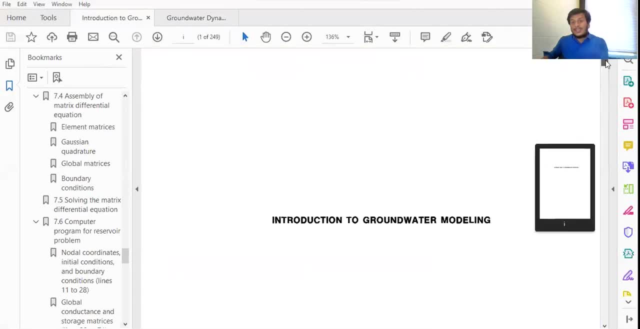 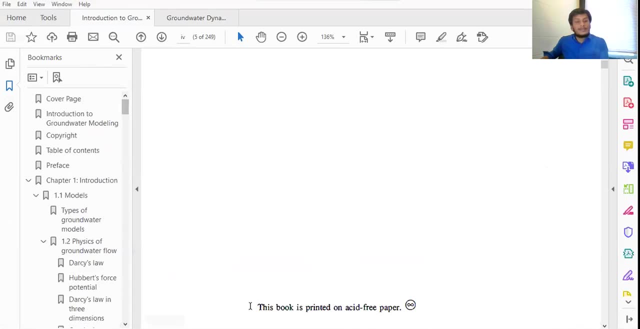 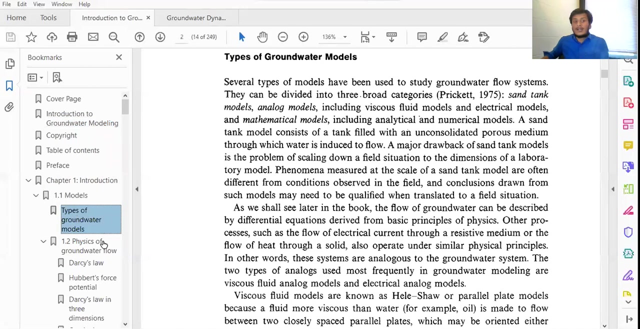 this study, few things related to. so this book, uh, i i got two books like uh which which are related, almost related to uh- partial differential equation. so so in this, in this book, like they try to explain the groundwater types of groundwater models and find a differential, how they 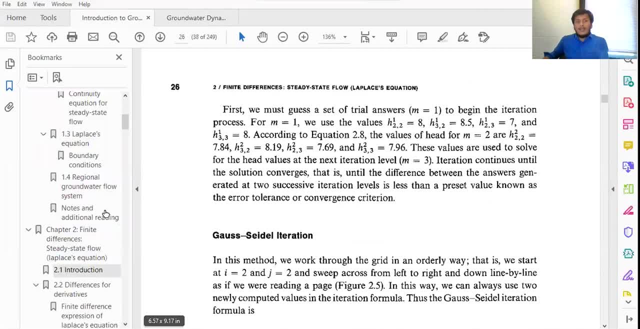 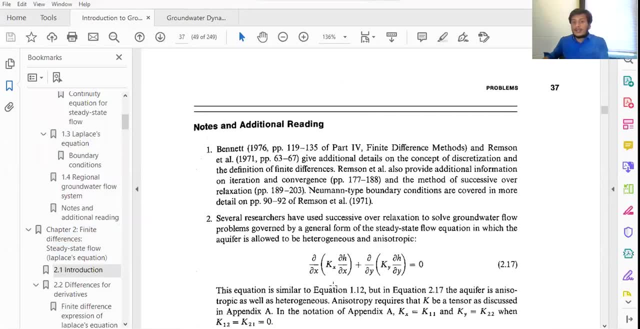 calculated the uh, they tried to sort out the equations, let's say this book. if you guys are interested to understand the in deep knowledge, like if you are interested to how uh, you know the, the, how they solve or sort it out. sort it out the partial- sorry, finite- difference model. 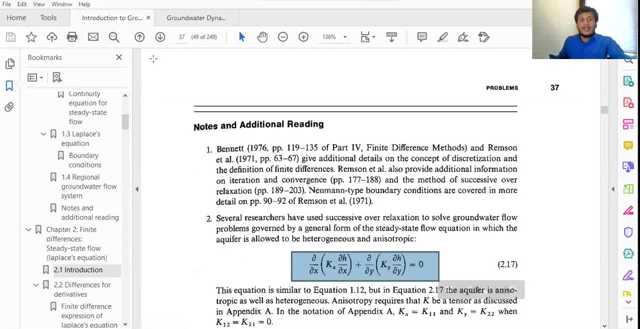 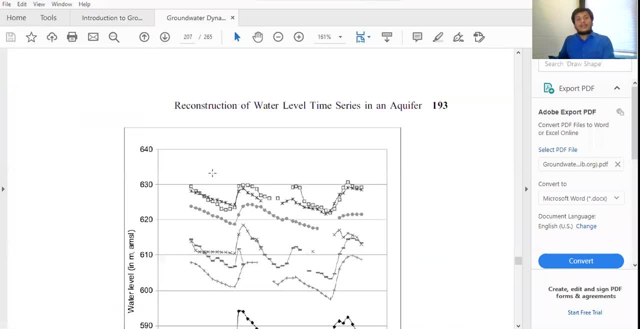 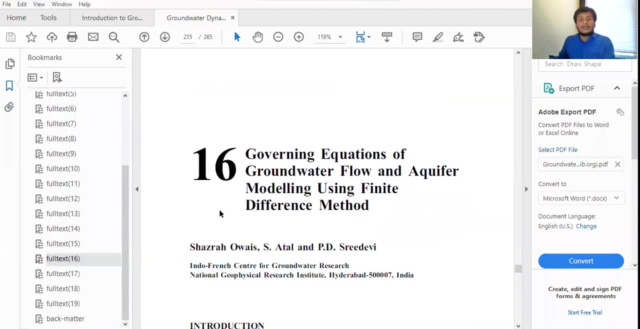 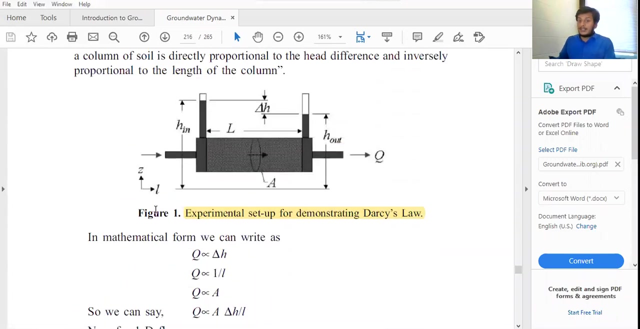 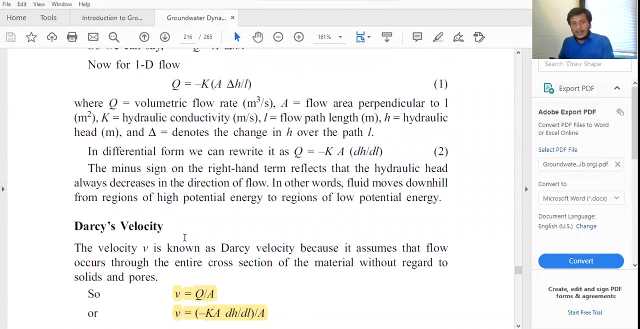 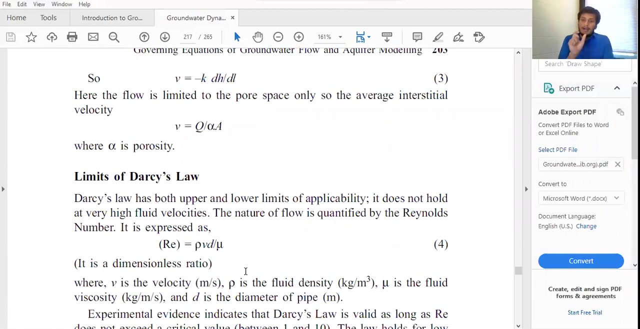 just, uh, i'd suggest this book and and the other one, like simply, yes, um, yeah, There's also Partial differential equation computer. so what they did was like they, you, They have used Darcy's law. We have solved this limit like v equal to qa. they use that. they try to initially, they try to make one small mass. 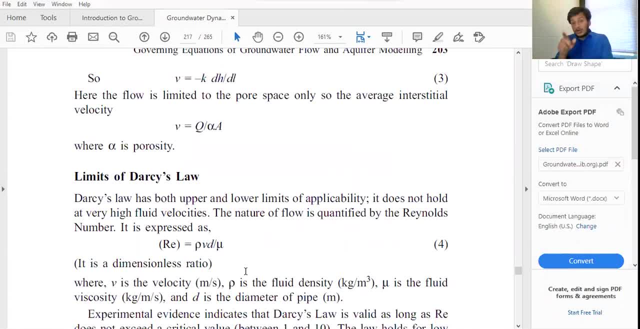 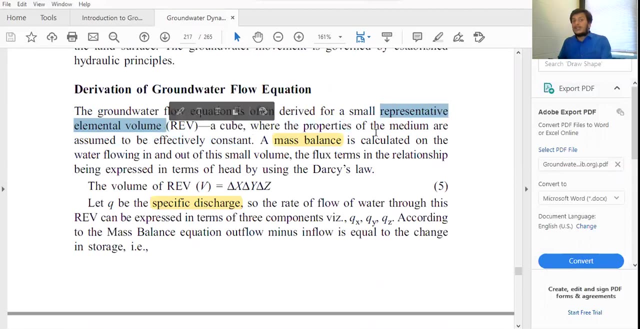 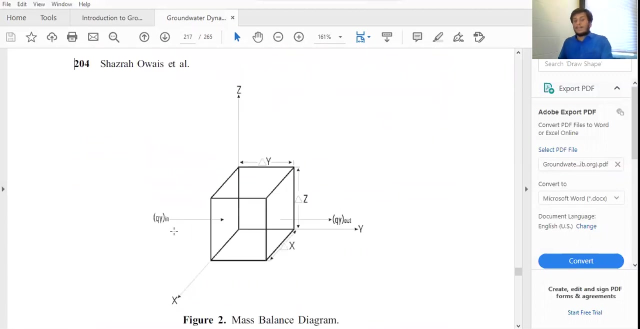 known mass cube to study the groundwater flow in that, in that queue, and they try to enhance to all the all over the area. so in this you would say, like rev representative element, elemental volume, like they try to study the mass balance calculated in the waterfall. so delta xyz is the volume of that's that are really representative elemental volume. then 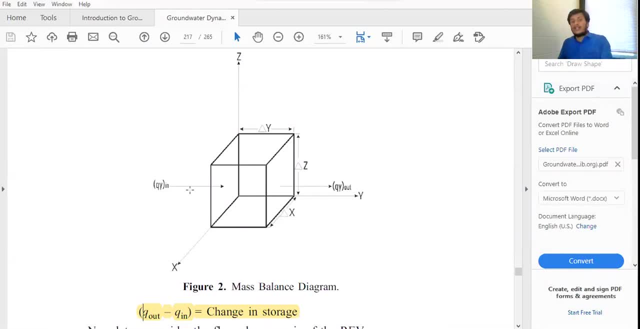 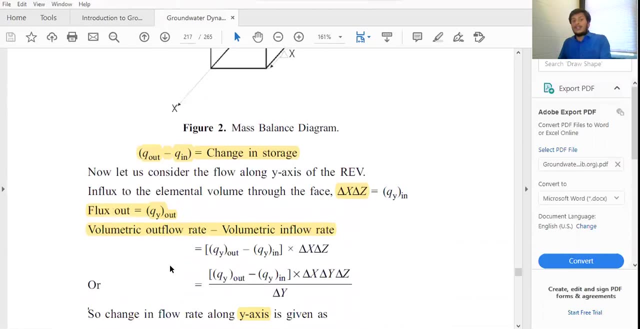 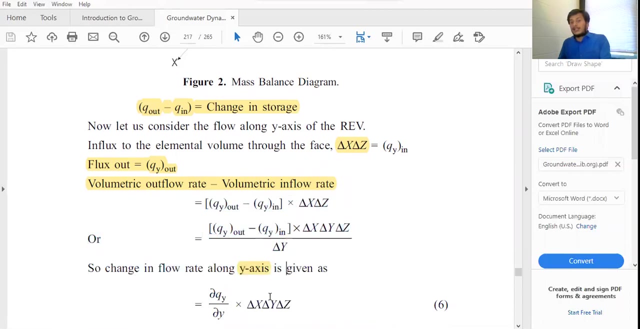 this is the representative of the dimension software and they calculate and they try to calculate the change in storage, q in and q out, discharge in, discharge out. so they try to sort it out in y direction, y axis, therefore this equation, similarly x and z axis. they got it. 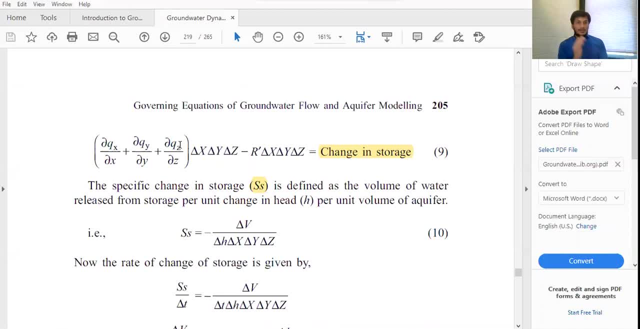 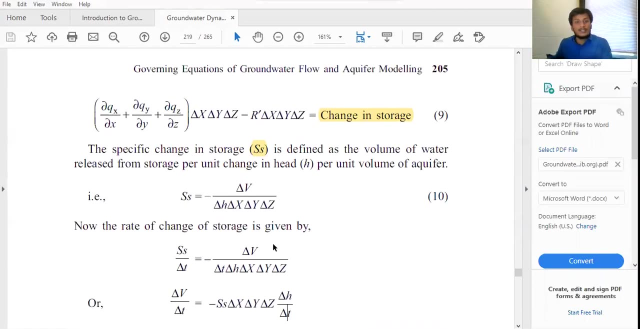 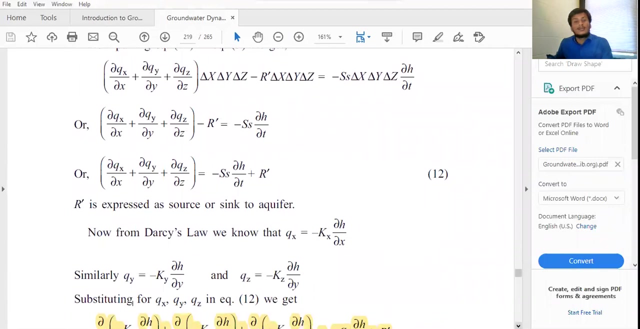 so slowly they try to. they try to include some other properties like conductivity, and all so slowly, slowly, one by one, one by one, one by one property. they're going to introduce them. they'll try to make a good equation beautifully, so they're going to get the final result. so this is the final equation, i would say finally, 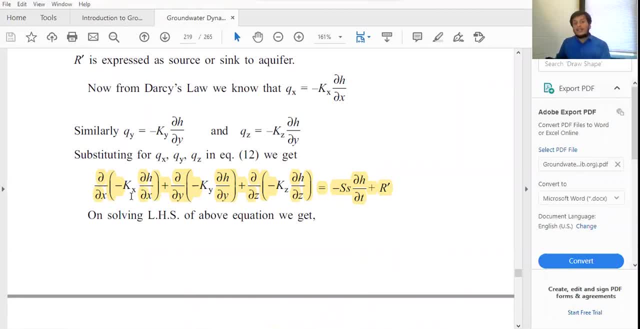 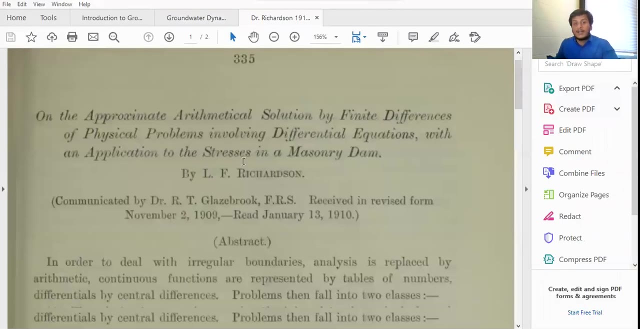 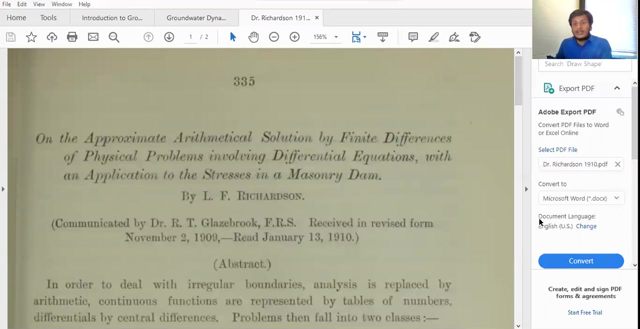 uh equation for the final difference equation that kx is the hydraulic conductivity, as we discussed in the presentation. that is how they got it. also, i got a few more articles. this is the first partial differential equation, 1910 i believe. so this, this, this article will help us if we're really 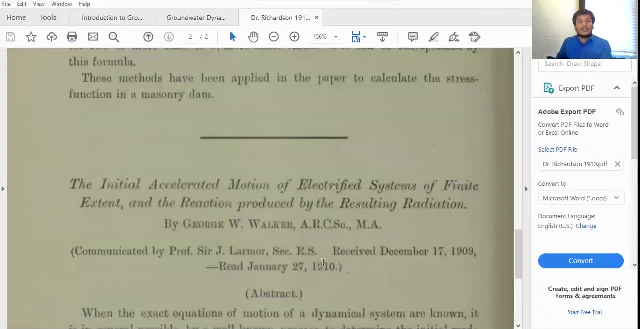 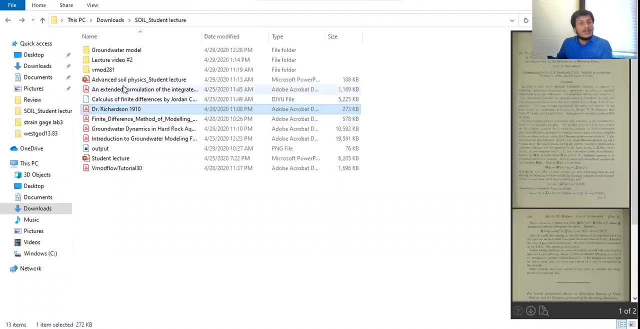 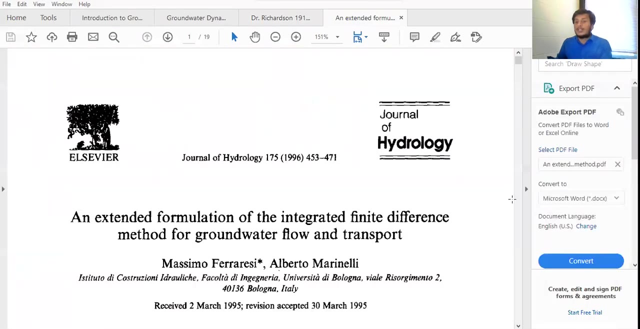 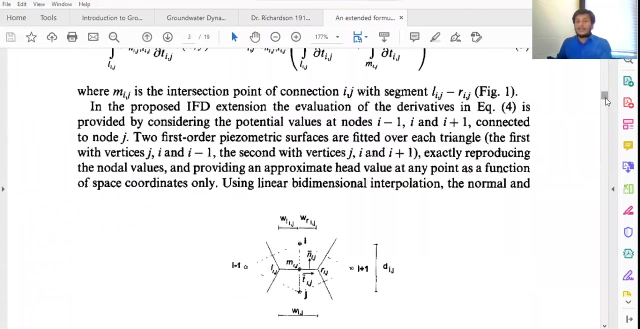 interested in this. this article would help us to how they worked on it and, yeah, an extended formulation of integration. i got some articles, so i'd like to share these articles to prove blackboard, if you guys want to like get this time to go through. yeah, coming back to the topic, yeah, 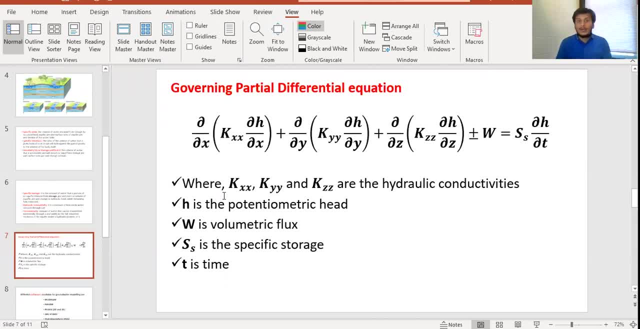 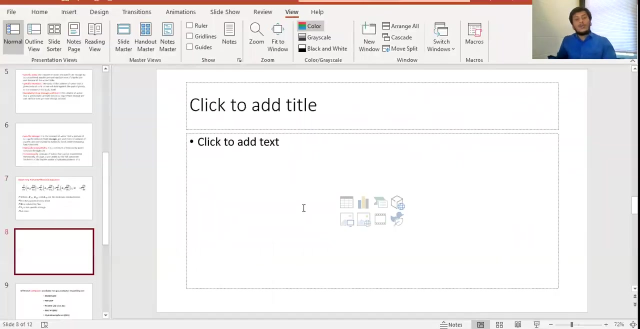 so that is how they they try to go and get the uh partial differential equation. so so, uh, coming to the groundwater flow modeling, before starting the software, i'd like to explain few more things. so we need to suppose let's discuss what. what are the uh data? we need to do the groundwater modeling. 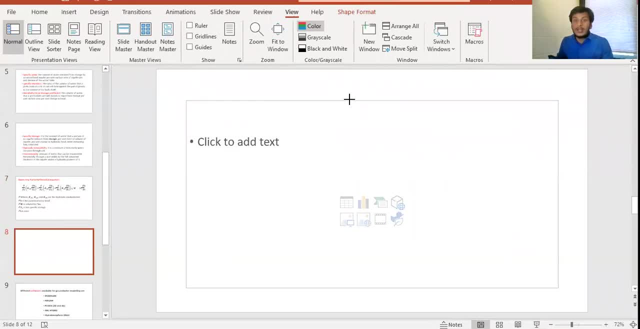 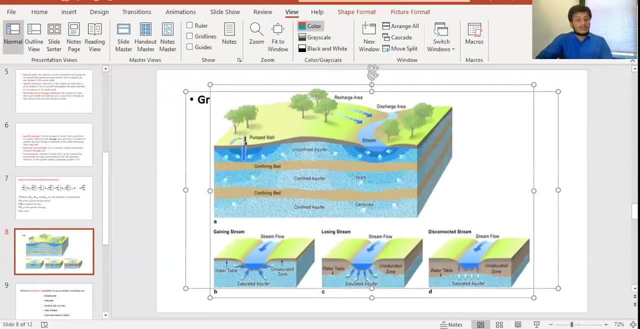 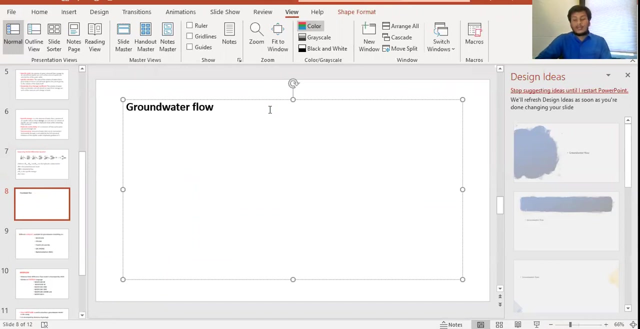 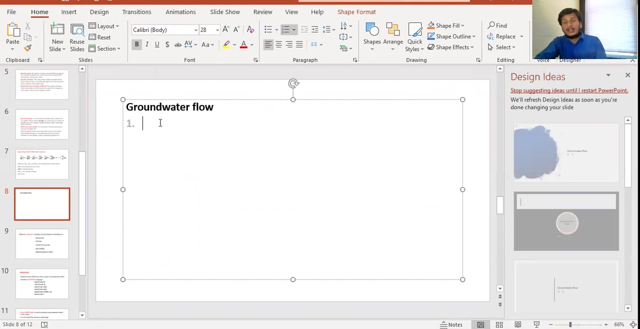 obviously we need. we need to model the groundwater flow. let us say we are going to do for far below, so we, through this, would be: yeah, let's say we are going to do for far below, so we, through this, would be: he r a data, so create a. 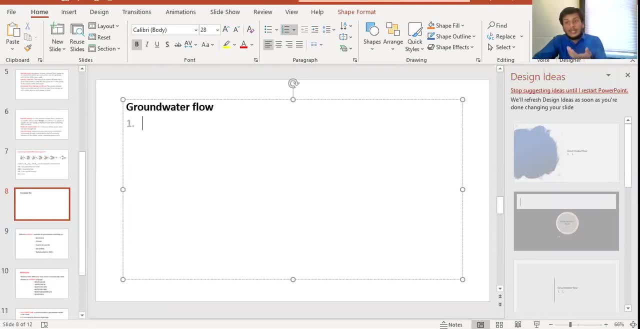 model in the, whereas uh in the in the visual model. what we need? a map, a map with its dimensions, dimensions or study area dimensions, dimensions of the study area, study area. it includes length and width. length and width of the dimensions. it could be in latitude, longitude or some. 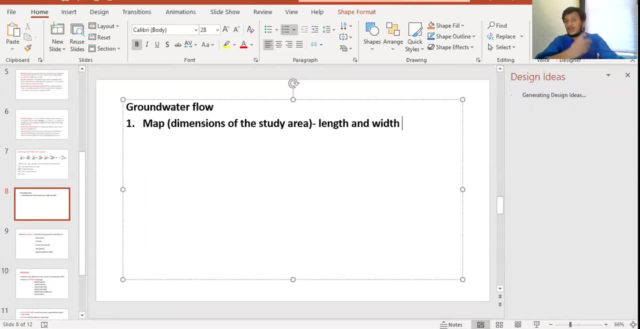 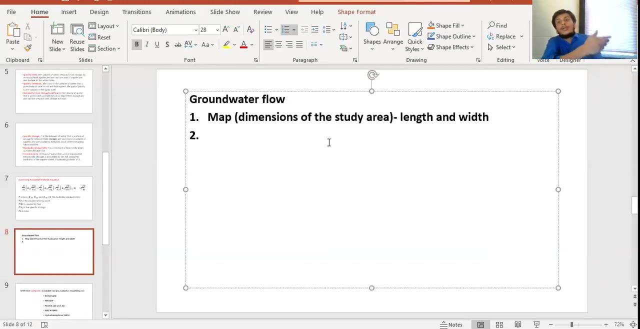 you know the uh. if you want to do in meters, you you're welcome to do that. yeah, we can doing that medical. then after getting the data, without elevation we are not going to monitor because visual outflow couldn't like get without any reference, it cannot say: this is the elevation at this. 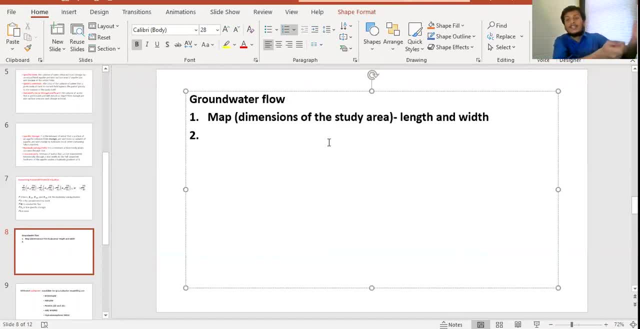 location. this is an elevation at the parking. this is elevation at the main door. this is elevation at the south entrance of faldo. it doesn't. so we need to view some reference points. so we need elevation. elevation in the science. uh, if we have more elevation, suppose if we say we got two part. 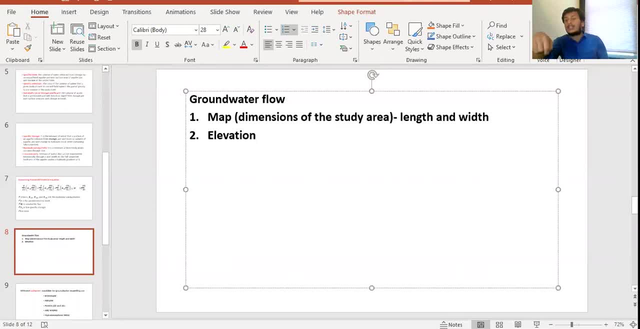 like elevation at north entrance and south entrance. if we ask the model to model will definitely do the integration itself and it will give the uh, it will allow the elevation. but it could be correct, it could be possibilities, chances are very less. so we need as many, as many, as many as locations. 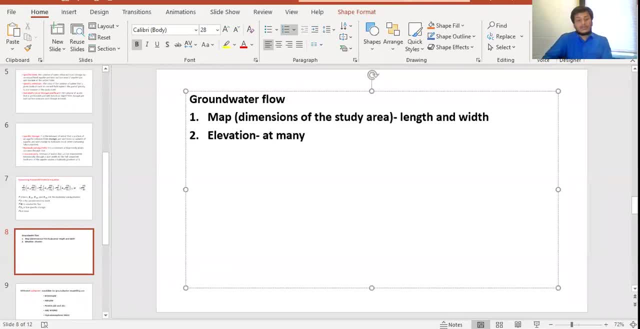 many, many locations. i'm forgetting evaluation. are we going to do like we got the elevation then goes to model the groundwater flow? we need? we need to know the real condition in the field. i mean, what kind of soil is there, how many layers are there, how deep it is? suppose if clay soil is around 10 centimeters, 10 meter deep if it is. 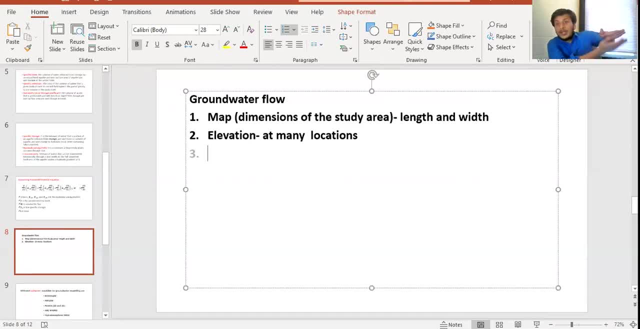 10 meter deep. then, from below the soil, clay soil, what's there? how deep you wanna wanna? wanna see how deep the ground water is. so, based on all these conditions, we need to know how many layers in the study area layers the study area into this clay, sandy soil. 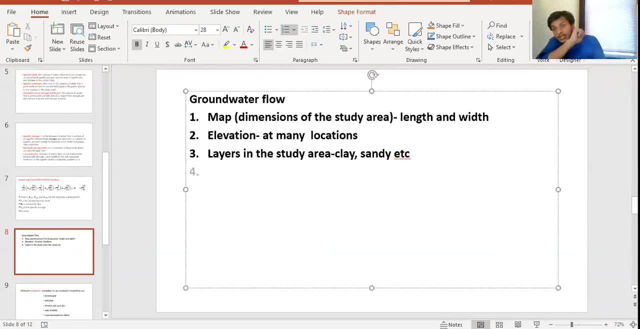 btc in soil, sandy soil, etc. then, uh, after getting this. so now we created the, the, the surface on the model. now we need, we are going to model the groundwater. it means we need some reference values of the existing observation values. so we need groundwater water. data could be from observation wells. 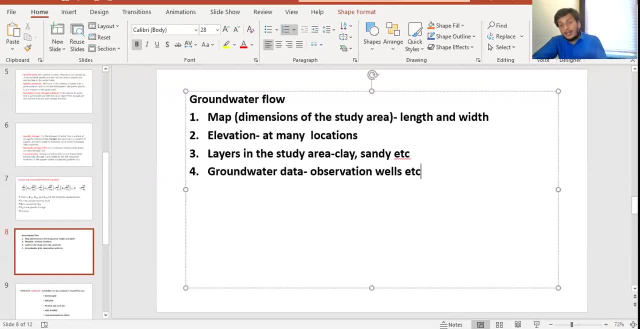 leaves, isometers, etc. how much data you need? as much as we can. if we have more data, the more accurately we can try to replicate the real condition. so that is how we do. so what else we need? obviously, if we have ground water wells, it's like. it's not like, only important there will be some, there should be. 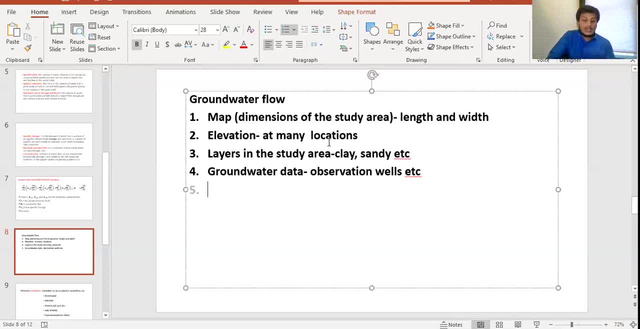 pumping wells in the Fargo Dome. We are going to say, if not in Fargo Dome, usually some countries use pumping wells to use groundwater. So usually we will be needing pumping wells. because if we don't have the pumping wells, that's fine. If we don't have pumping wells. 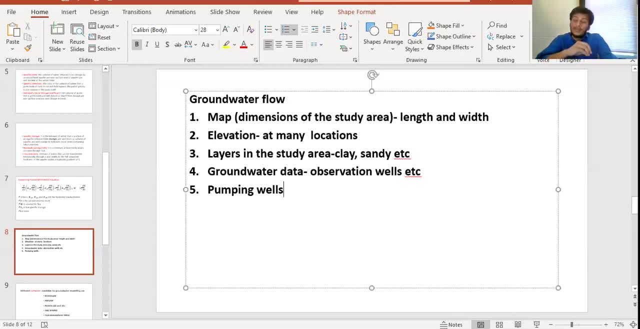 in real condition. that's fine. But if we have pumping well data and if you are not going to assign them in the model, then obviously there will be like possibility of we are not going to create real conditions. That means obviously we need- at least we should- 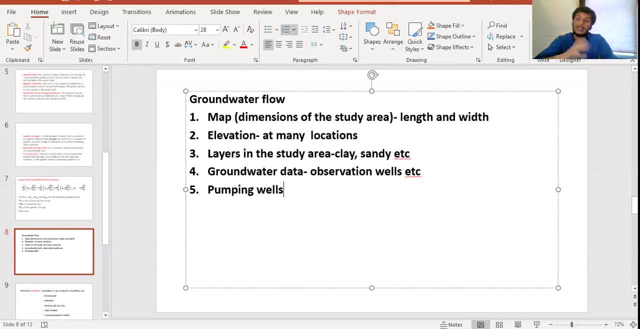 get. try our best to find the pumping wells and get the data. How much data we need? Obviously, yes, How long? Like as much as you can? Yeah, Then, after the pumping wells, what do we need? So we need properties, Properties of the 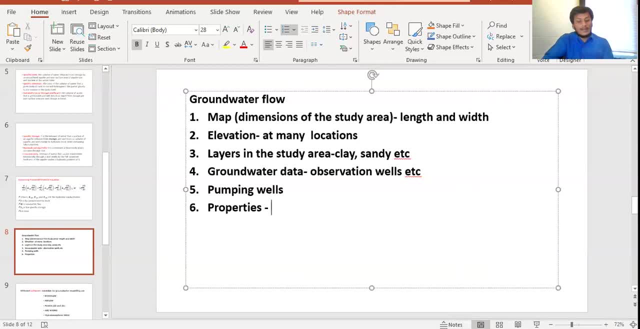 Layers Like hydraulic conductivity, specific storage, total porosity, ETC, total porosity, porosity, porosity. These are the. these are the important functions properties. Yeah, These are the important properties, So which we need to know. Also, we need the layer thickness. 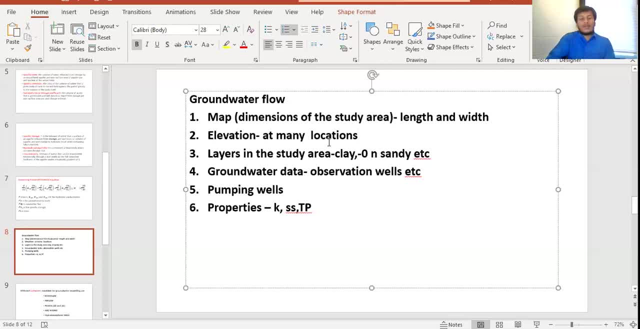 Number of layers. Number of layers, The thickness of each layer, Thickness of each layer, These also, these are like a bit important for our model. So after getting the pumping wells, we need to assign the support alone. We are almost. 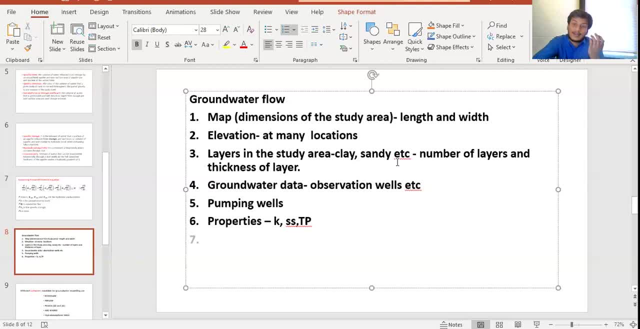 about to get there. So now we need rivers, like surface water, boundaries, Boundary conditions. we need to get- If you have a sea or ocean, say, river lineage, canals, Some kind of boundary conditions. boundary conditions, boundary conditions like c, it should say like zero head. 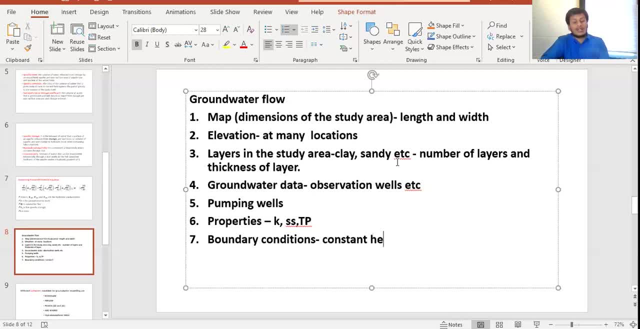 constant head would say constant head. it comes under portion of c. yeah, c would be like zero. is the mean sea level? right? that's what i mean and reverse. can i say that canals mean drainage canals? nine canals, i mean you cannot start smaller. we were like which would have the things which would have impact on. 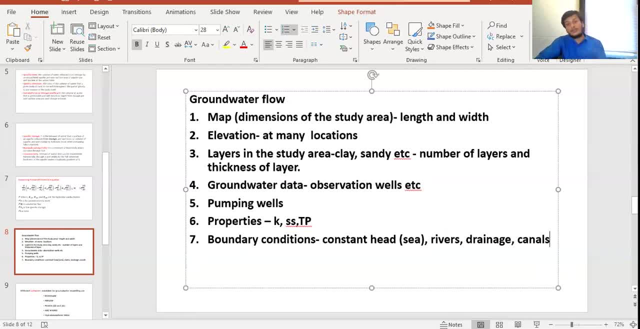 the groundwater, that those are all like things we need to do. then what else we need? we need to know the evapotranspiration if we are going to do in the field, average evapotranspiration, how much data we need, how much we can. this big story like: uh, then recharge, recharge is the 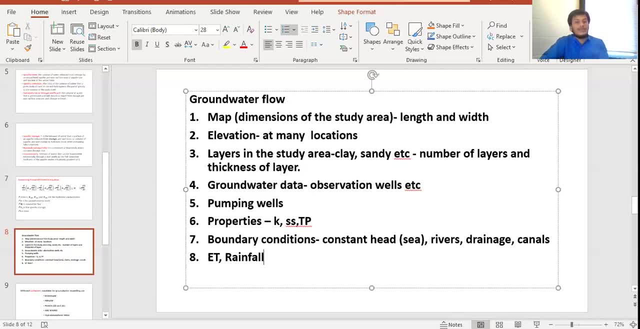 rainfall, we have rainfall, right. so we'll say i uh this, usually, if we don't know how much research, we'll say 10 percent of the rainfall, annual rainfall year. these are like 10 percent of the rainfall, i believe i. i try to explain almost all the the inputs for the model without